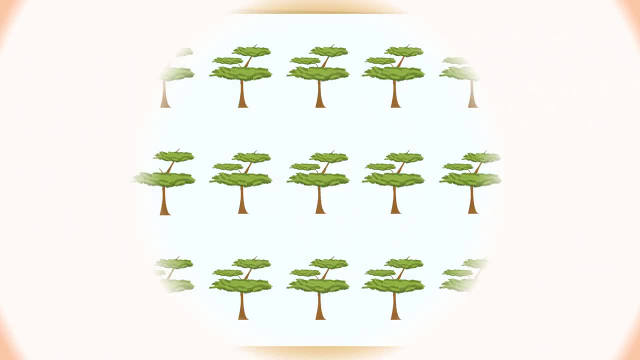 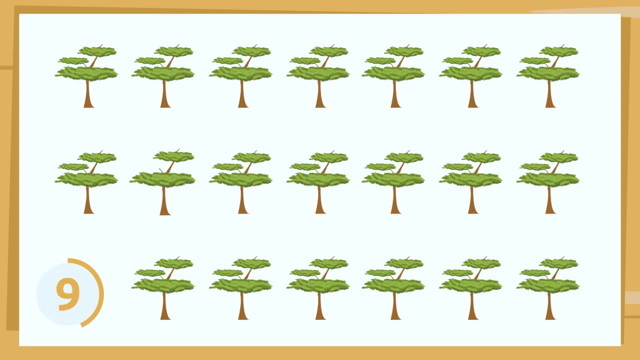 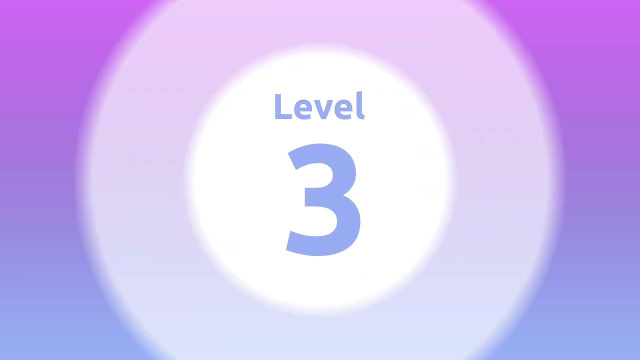 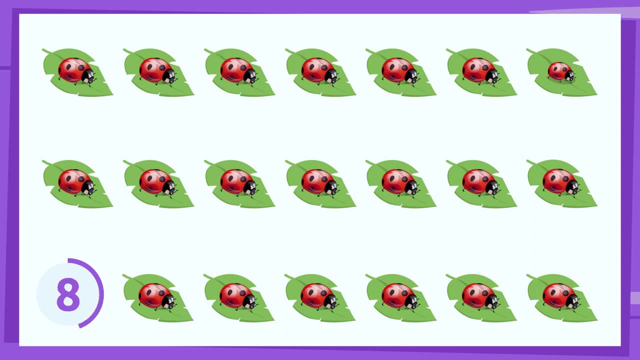 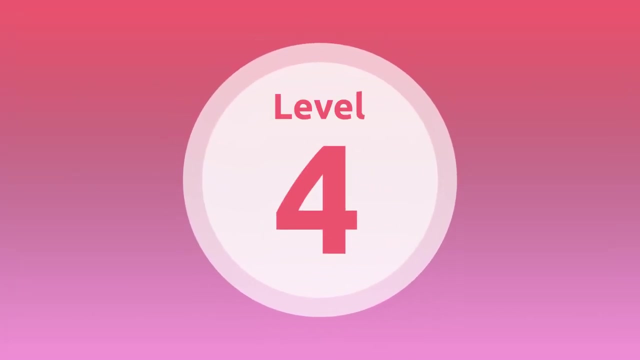 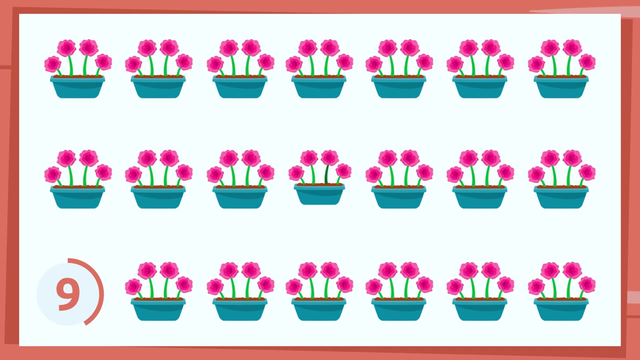 Level 2: Can you see it Right here? Easy, right. Let's see how you do with the next one, Level 3: Where is it Right here? Let's do the next one, Level 4, And the different drawing is right here. I'm sure the next one is not as easy. 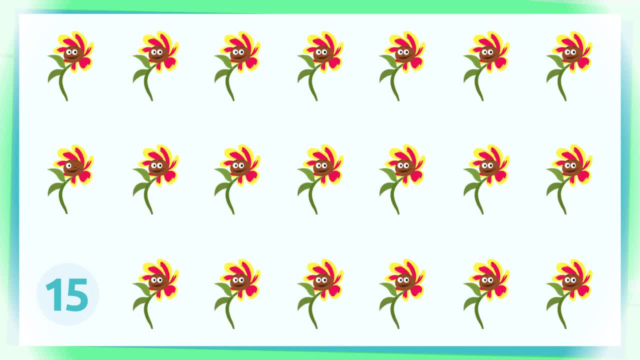 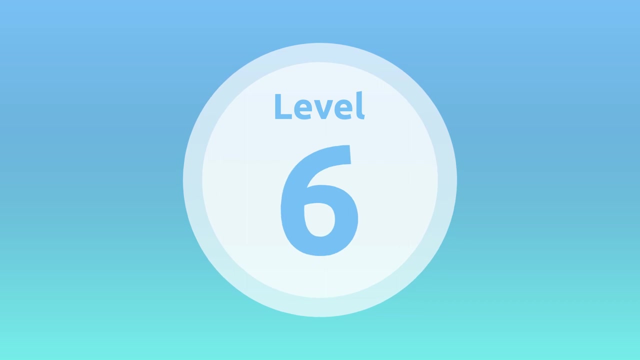 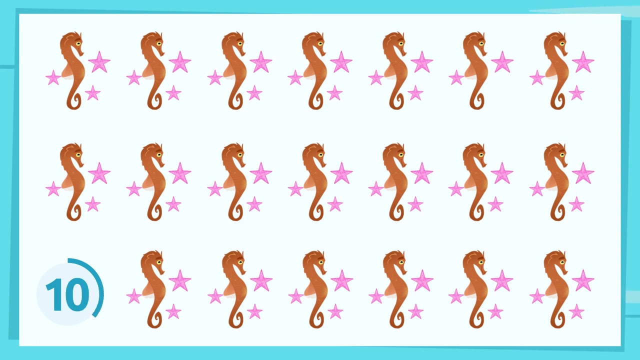 Level 5: This is getting complicated. It's right here. Don't drop off to sleep, Let's do another round. Level 6: This is getting complicated, It's right here. Don't drop off to sleep, Let's do another round. 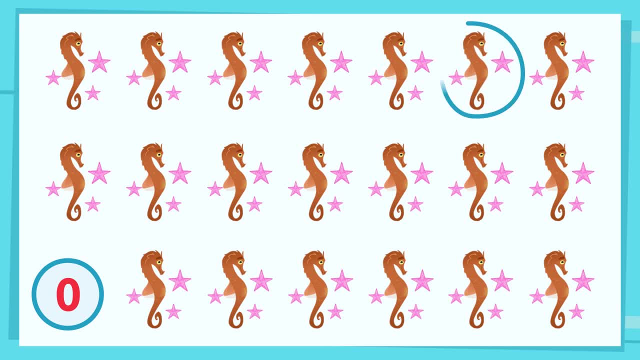 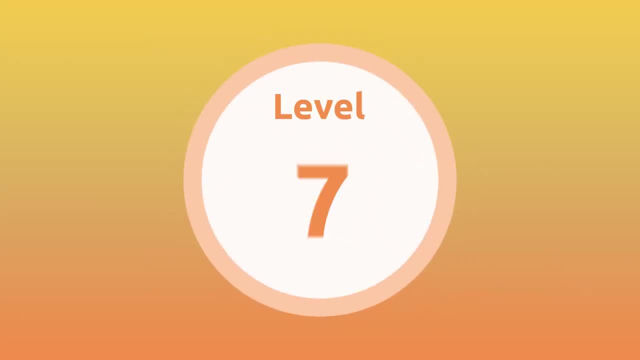 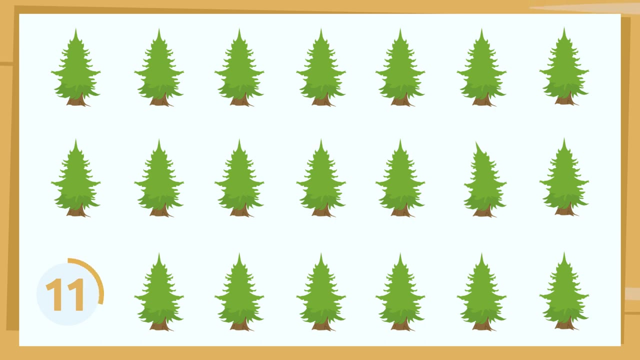 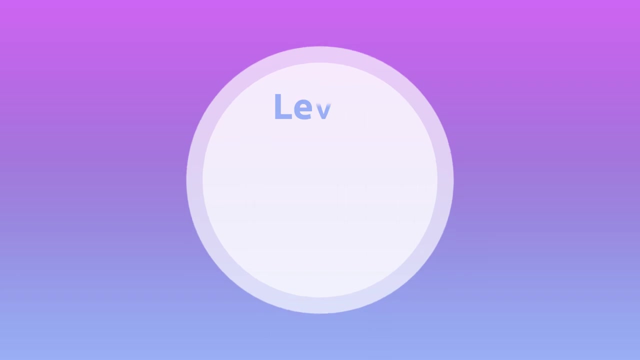 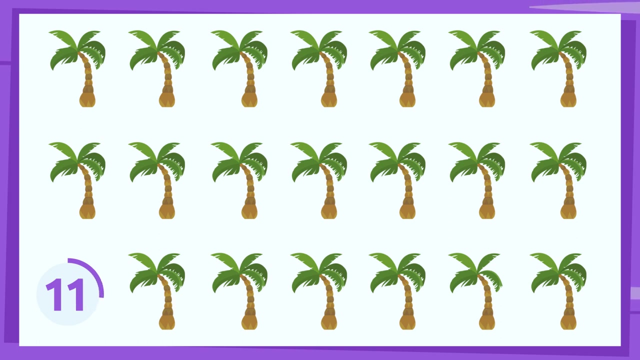 Have you spotted it? Here it is. There are a few levels to go. Level 7: This is getting complicated, It's right here. Don't drop off to sleep, Let's do another round. Level 8: This is getting complicated, It's right here. Don't drop off to sleep, Let's do another round.